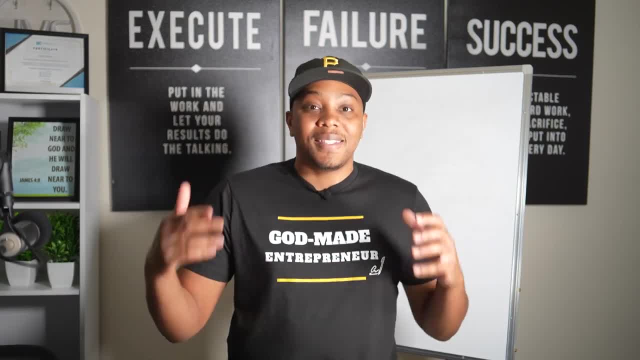 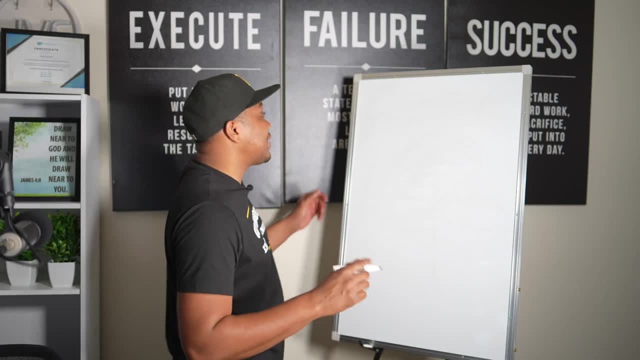 explanation and so that you can get one step closer to making a consistent stream of income trading in the foreign exchange market. Let's get into it Now. as always, I got to have my whiteboard, So let's get into it. What are you looking at when you look at a Forex chart? So, 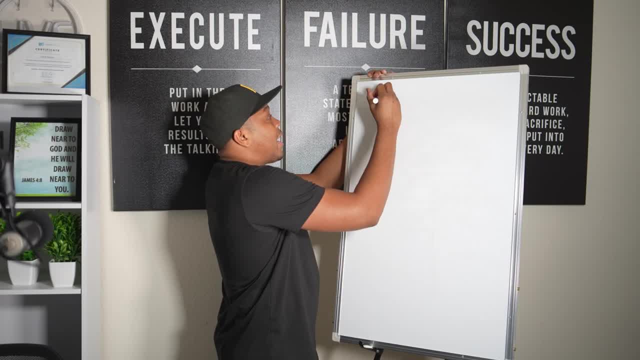 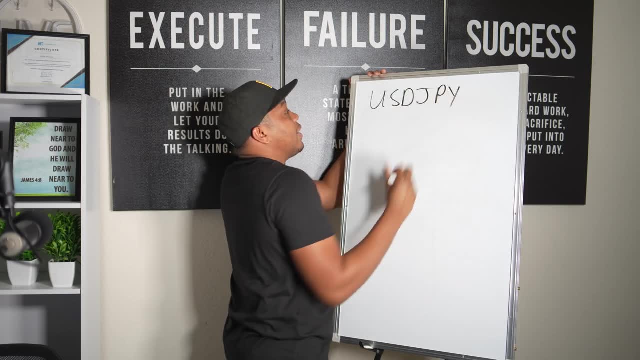 let's just say, for instance, like I said in my first example, you're looking at a chart that says USD and you see right next to it, JPY. okay, Now, this will be a pair that we like to call UJ, okay. 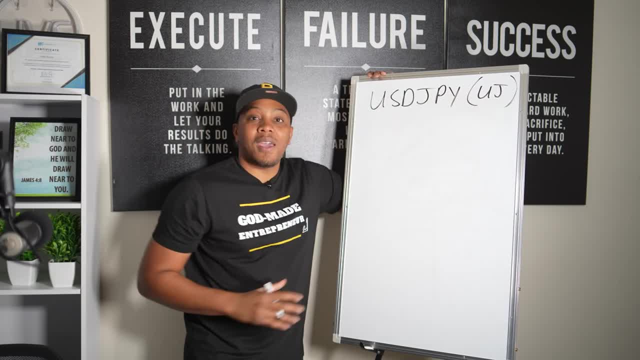 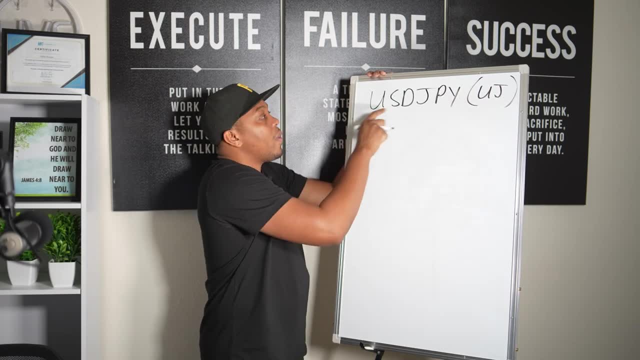 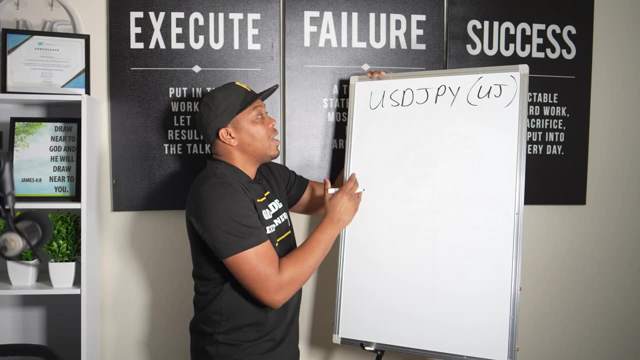 Now, what does this stand for? first, Before we even get into what we're looking at in the chart, what does that stand for? Well, basically, what this stands for is: USD stands for US dollar, JPY stands for Japanese yen. okay, So this is the US dollar compared to the Japanese yen, That is. 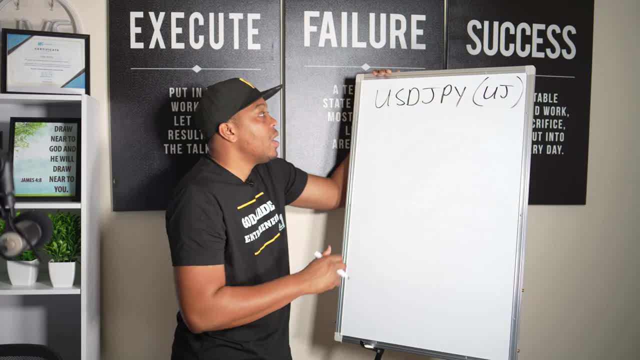 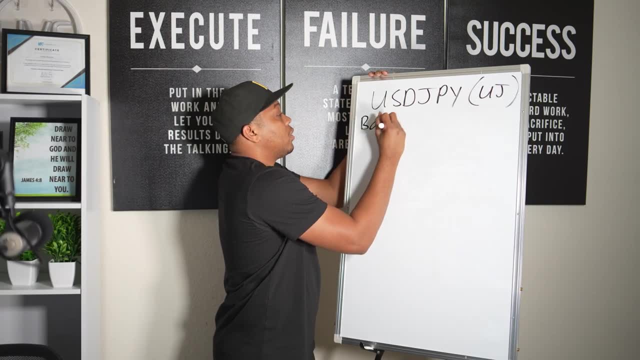 what this currency pair represents and that's what this stands for. Now, when we look at currency pairs and when we're looking at a chart, you got to understand that we have two things. We have what's called a base- okay, And then we have what's called a quote- okay, You have a base. 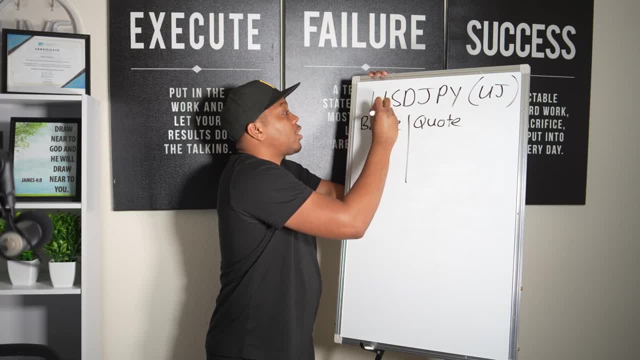 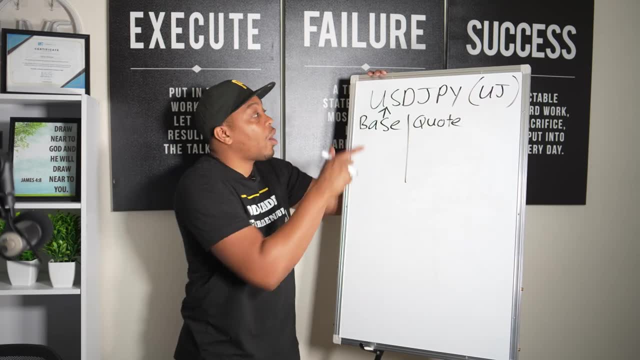 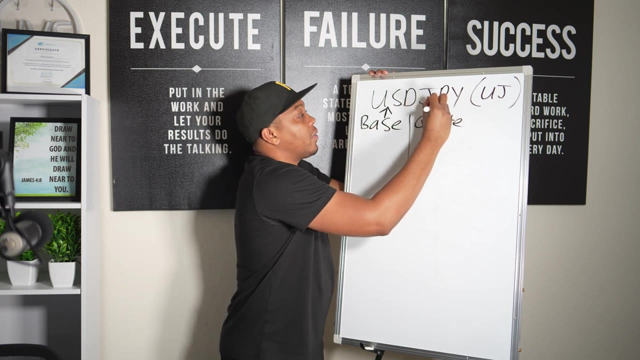 and you have a quote: The base is always the first currency in a currency pair. okay, So when you look at a currency pair, you're going to have two currencies that are compared side by side. The first currency in that currency pair is going to always be your base, The second currency in that. 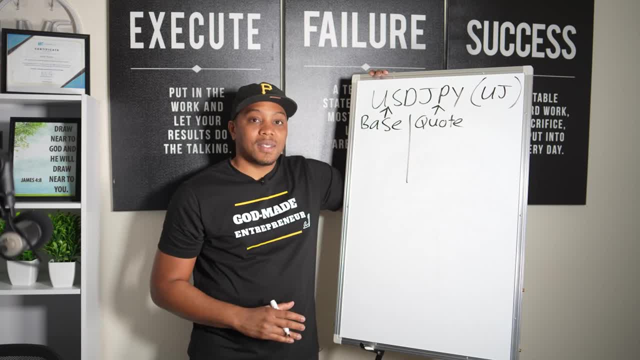 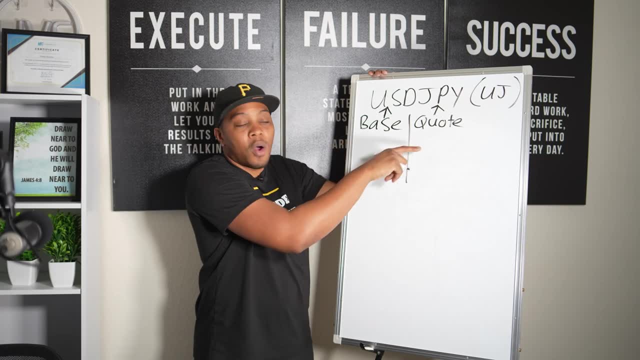 currency pair is going to be your quote. Now, why does this make sense When we're looking at a chart, a Forex chart? simple, I'm going to tell you right now: When the base is stronger than the quote, typically the chart you're looking at is going to be. 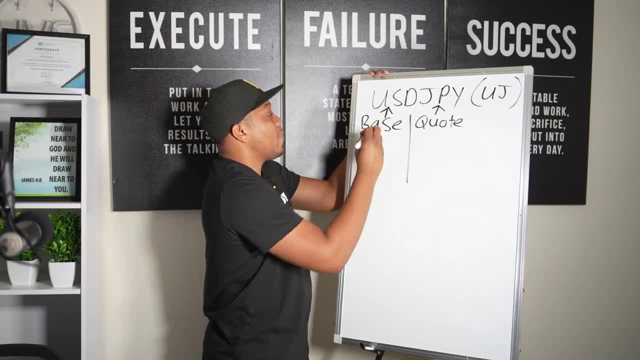 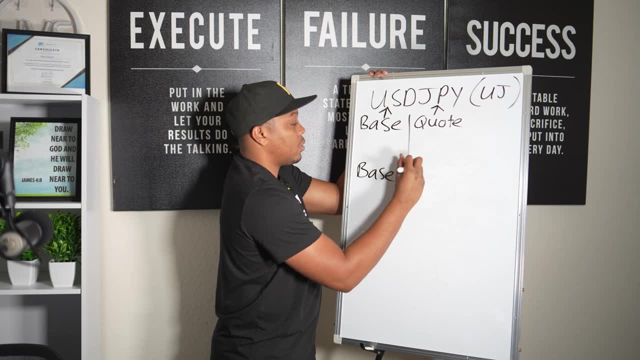 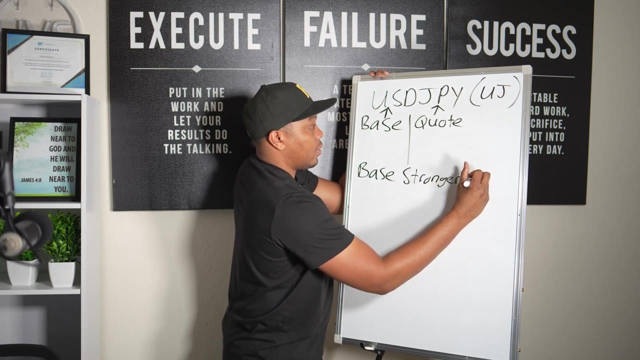 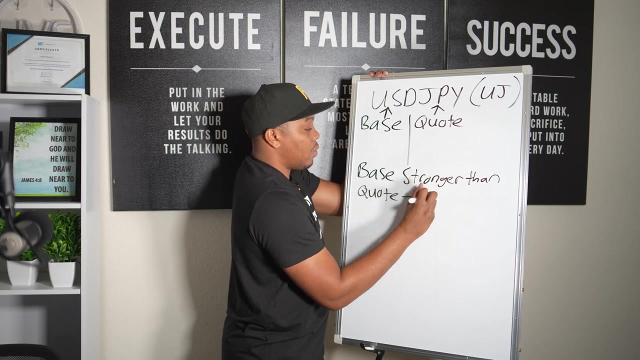 trending in a upward direction. okay, So again, when- and we'll just put this right here- okay, We'll put base stronger in a upward direction. okay, Then quote: you're going to see price trending up. okay, So you're. 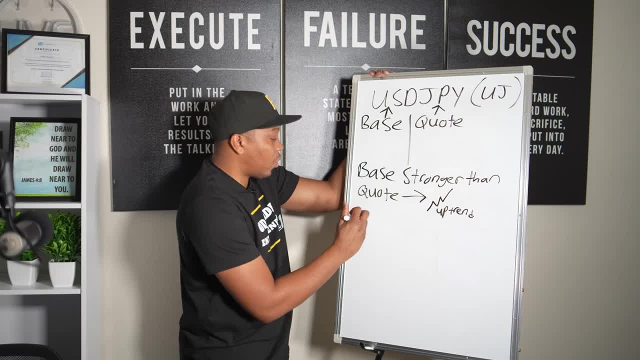 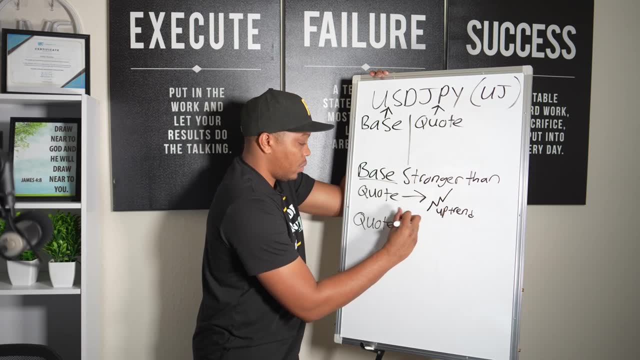 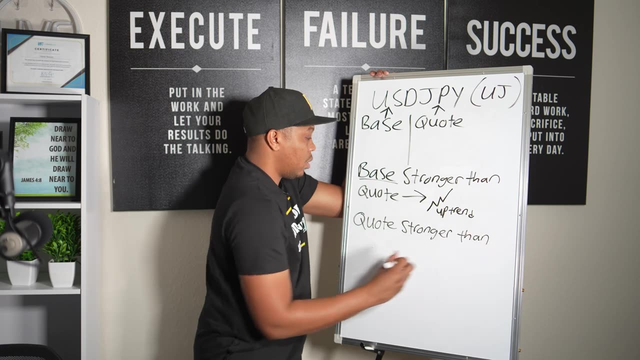 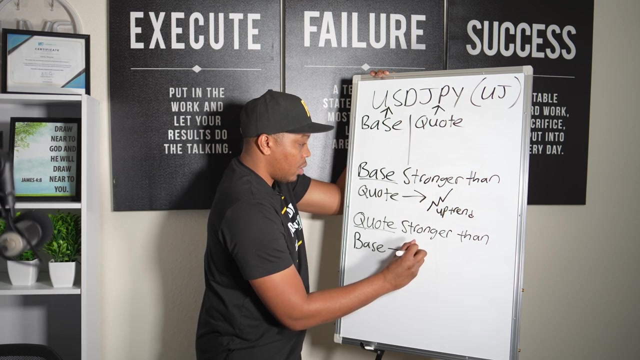 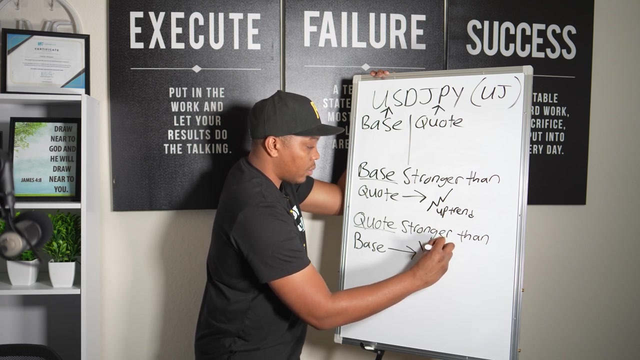 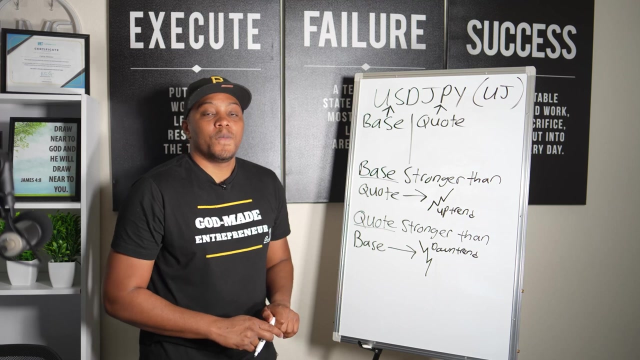 going to be looking at an uptrend all right Now when the quote is stronger. when the quote is stronger then the base, you should be seeing a downtrend on your chart. okay, And this is how you understand what you're looking at when you're looking at a Forex. 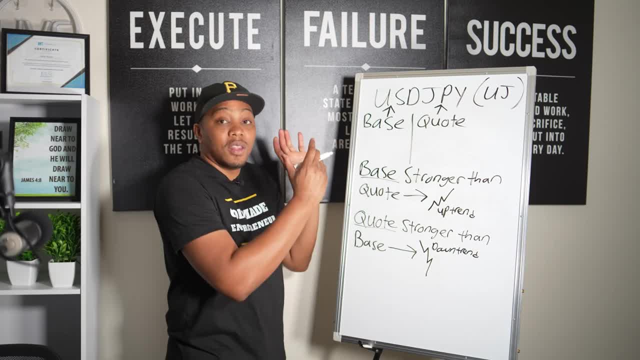 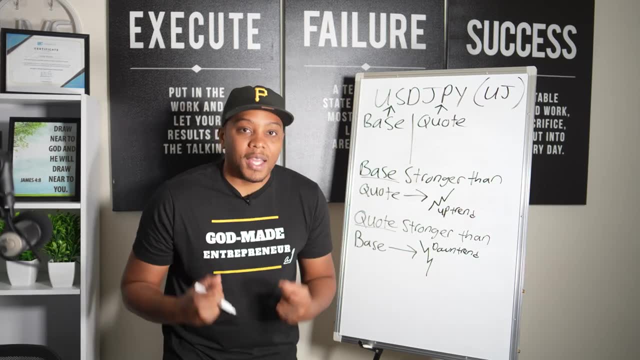 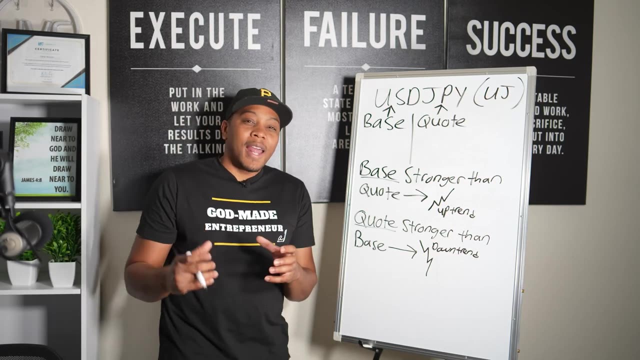 chart, Okay. By simply understanding the currency pairs and understanding the base and the quote of that currency pair, this can give you a better understanding of what you're looking at. when you're looking at a actual Forex chart, Okay. Now the next thing is when you're looking at a chart. 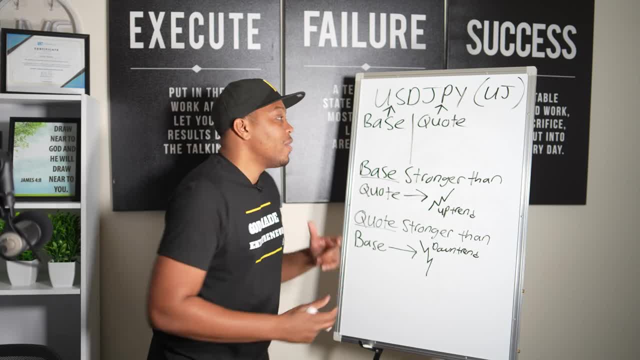 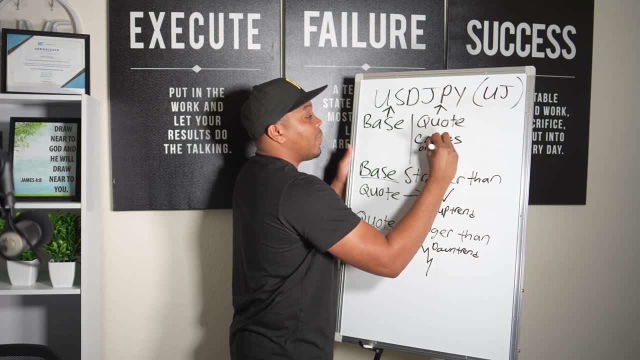 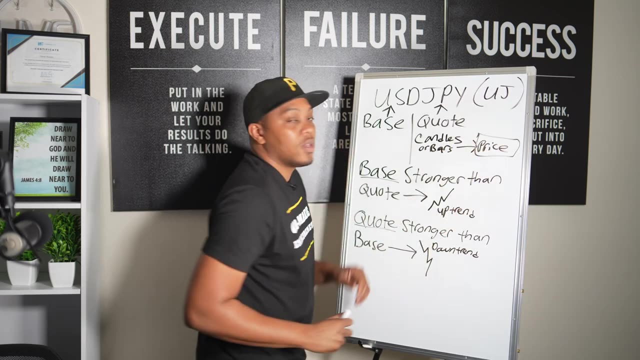 and you see those candlesticks or you see those bars- Okay. So when you see candlesticks, all right, candles on your chart or bars moving up and down, Okay, This represents price. Okay, This represents price. So when you open up your chart and you're looking and you see these, 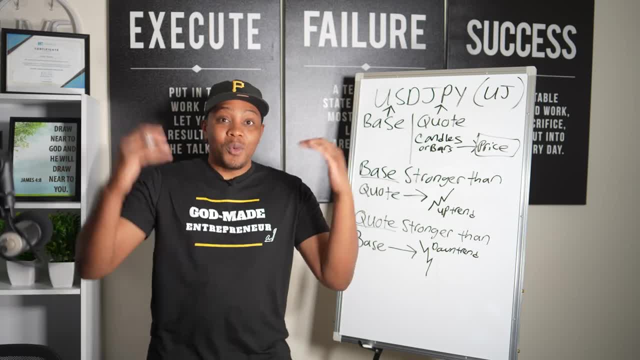 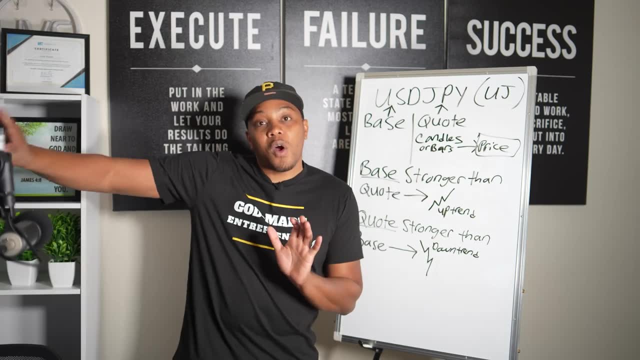 bars or candles, whatever you call it right now. right, And you see it moving up and down. that's representing price. Price is moving, Price is fluctuating. And if you look on the far right side of your chart, if you're looking on tradingviewcom- 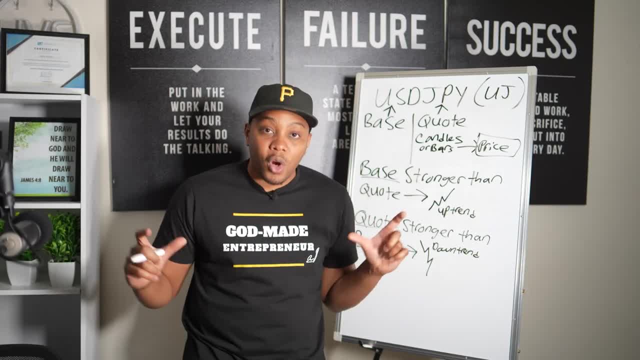 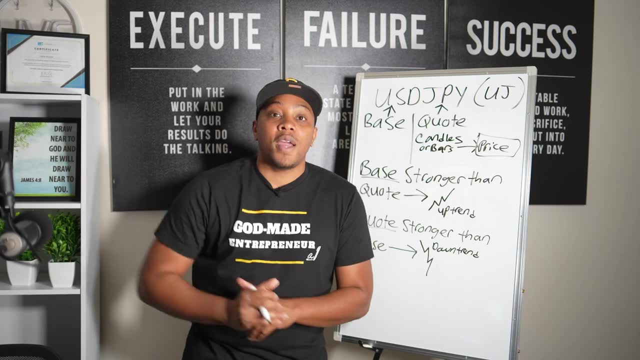 which is the site that I recommend that you can use for your charting. that's where you can actually look at charts And that's where you can actually view your different currency pairs. If you look on the far right of your trading view chart, you'll see numbers. All right, You'll see. 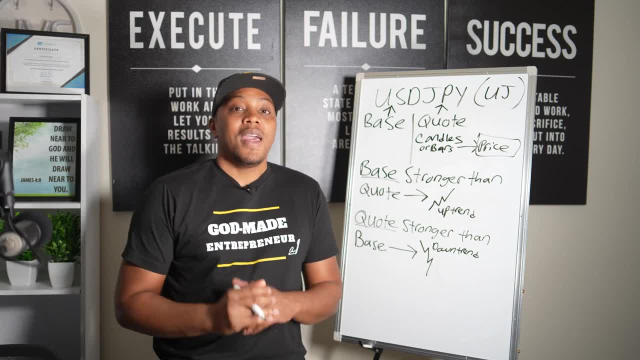 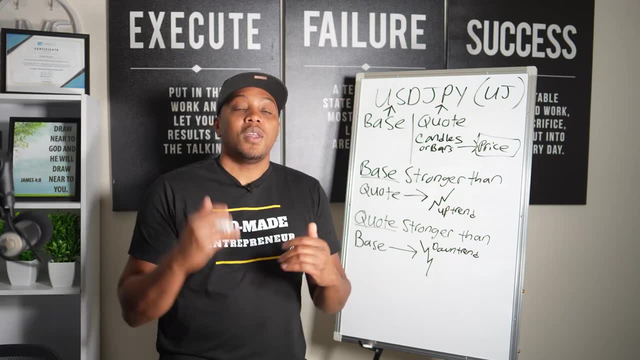 numbers from the top to the bottom on the far right of your chart, And that is going to represent the actual price numbers And you're going to see those candlesticks moving in between those prices, showing you the fluctuations in price as business is taking place. All right, So now, once you 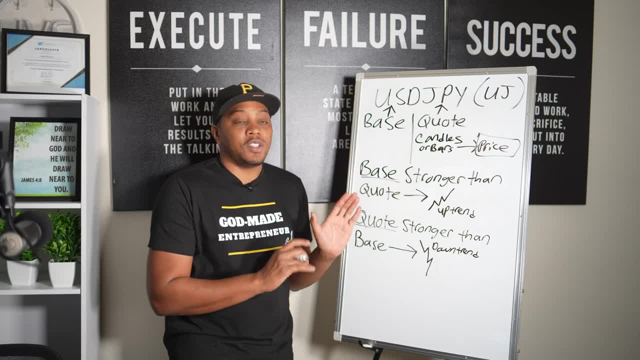 understand the basis of the chart, you're going to be able to see the price numbers. So when you understand the base, you understand the quote. you understand the candlesticks. you understand the bars on the chart. they represent price moving. All right, Business being taking place.